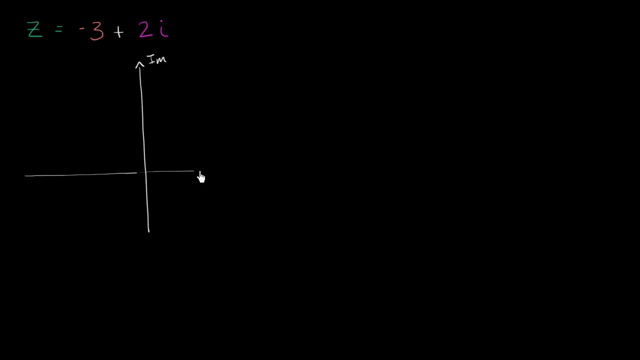 imaginary axis and that is our real axis. real axis- and let's see the real part- is negative three. so we could go one, two, three to the left of the origin. Let me space that out a little bit more evenly. 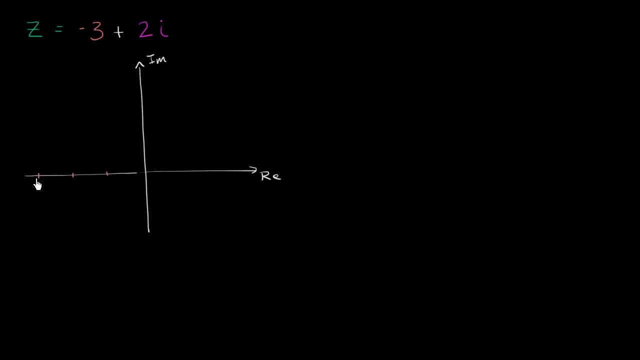 So one, two, three to the left of the origin, so negative three. and then we have two i's, So we're gonna go up two, so up two in the imaginary direction. So one, two, just like that. 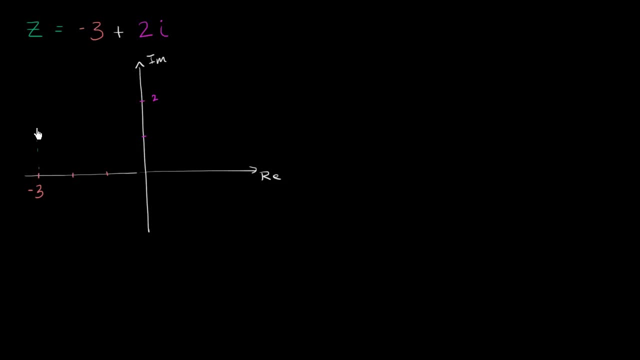 And so z is real part negative three, imaginary part two: z would be right over here in the complex plane, So that is z, right over there. Now what I wanna think about are other ways to essentially specify the location of z And in particular, instead of giving the real 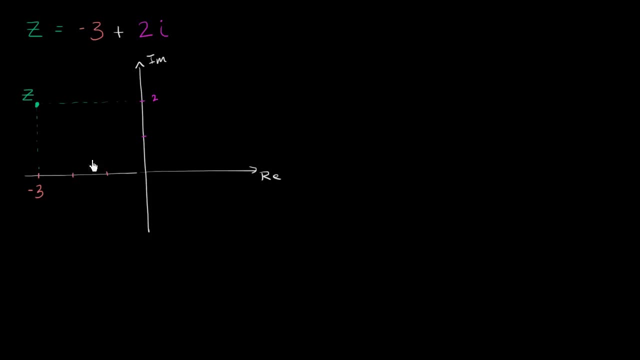 and imaginary parts, essentially the coordinates. here let's think about giving a direction and a distance to get to z. So for example, we could give the distance from the origin to z. So let's call this distance r. But that distance by itself isn't enough. 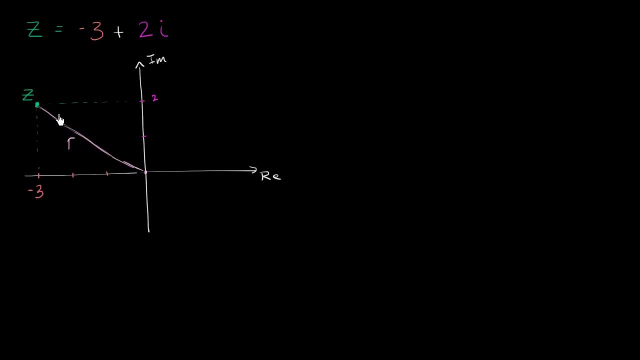 to say where z is, You have to say in what direction do you have to go a distance of r to get to z, And so to specify the direction. to specify the direction, we will have this angle, theta in radians, this angle between the positive real axis. 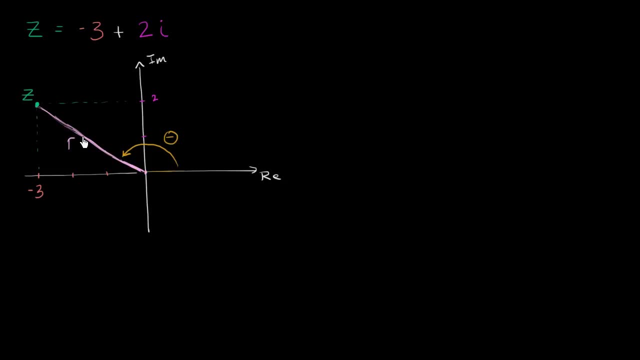 and this line right over here, this line or this segment that connects the origin and z. So if someone gave you this angle and this distance, then you could get to z Now, what I want you to do right now is pause this video and see if you can find. 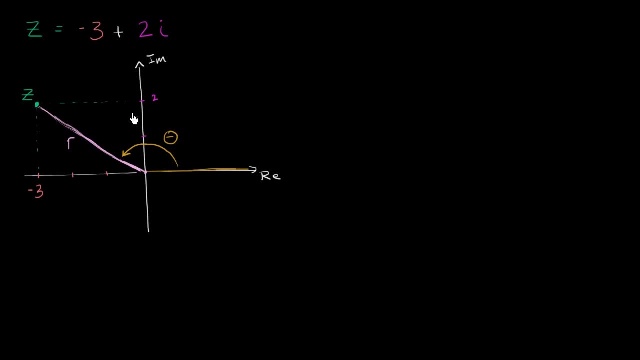 a relationship between r, theta and negative three and two. In fact, given this complex number in rectangular form, can you figure out what r and theta are? Well, let's think through this a little bit And, to help us with that, let's remind ourselves. 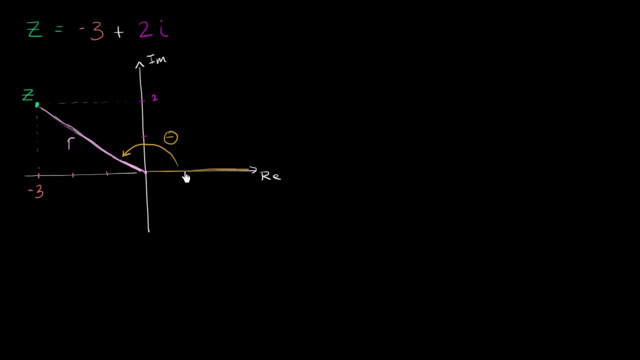 of the unit circle. definition of trig functions. because we are going to use some trig functions to relate r, theta and two and negative three. So I'm gonna construct a unit circle here. So construct a unit circle. So this right here is a unit circle. 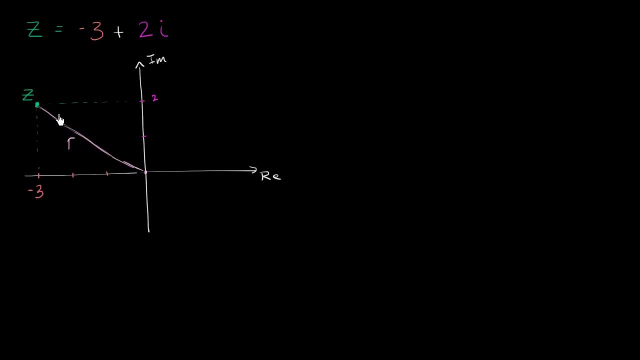 to say where z is, You have to say in what direction do you have to go a distance of r to get to z, And so to specify the direction. to specify the direction, we will have this angle, theta in radians, this angle between the positive real axis. 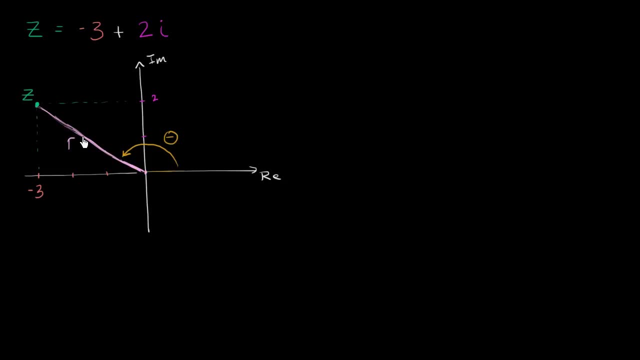 and this line right over here, this line or this segment that connects the origin and z. So if someone gave you this angle and this distance, then you could get to z Now, what I want you to do right now is pause this video and see if you can find. 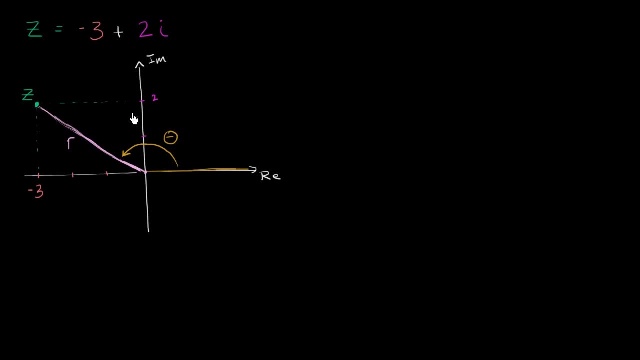 a relationship between r, theta and negative three and two. In fact, given this complex number in rectangular form, can you figure out what r and theta are? Well, let's think through this a little bit And, to help us with that, let's remind ourselves. of the unit circle. definition of trig functions. because we are going to use some trig functions to relate r, theta and two and negative three. So I'm gonna construct a unit circle here. So construct a unit circle. So this right here is a unit circle. 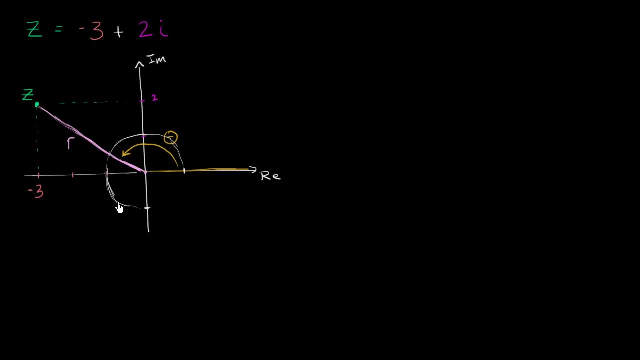 circle of radius one. So construct a unit circle. That's a unit circle By definition. what are the horizontal and vertical coordinates of this point right over here, Where this line intersects the unit circle? Well, this is forming an angle of theta. 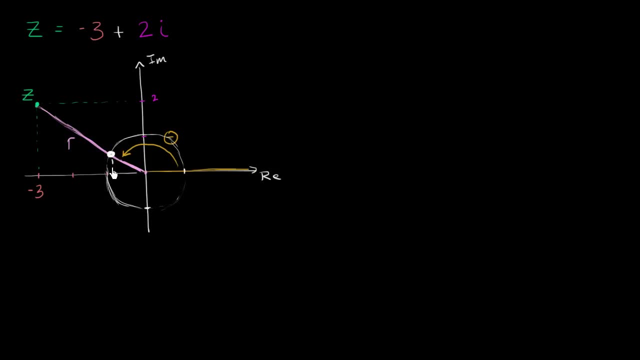 with a positive real axis, And so the horizontal coordinate over here by definition is going to be cosine of theta, cosine of theta. That's the unit circle definition of cosine of theta, And the vertical coordinate is going to be cosine of theta, cosine of theta. 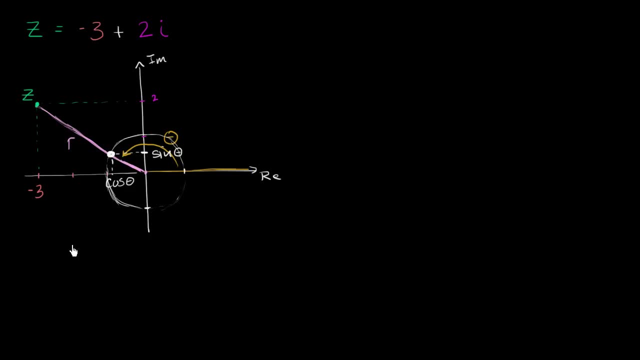 So there you go. That's the unit circle definition of cosine of theta to be sine of theta, sine of theta. And so what would the horizontal and vertical coordinates of this point be? We obviously know they're negative three and they're two. 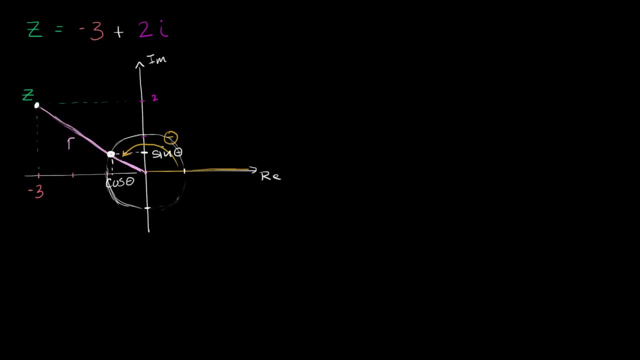 but what would they be in terms of cosine theta and sine of theta? Well, look, this point right over here is a radius of one away from the origin. So this distance right over here, that distance right over here, is one, But now we are r away from the origin. 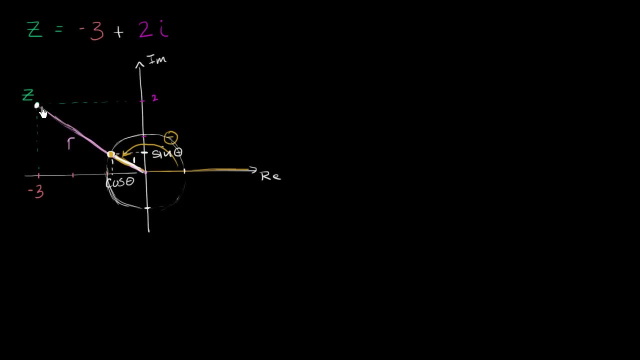 We're r times as far, So for r times as far in that direction, then we're going to be r times as far in the vertical direction and r times as far in the horizontal direction. We're gonna have to scale all of. we're gonna scale everything by r. 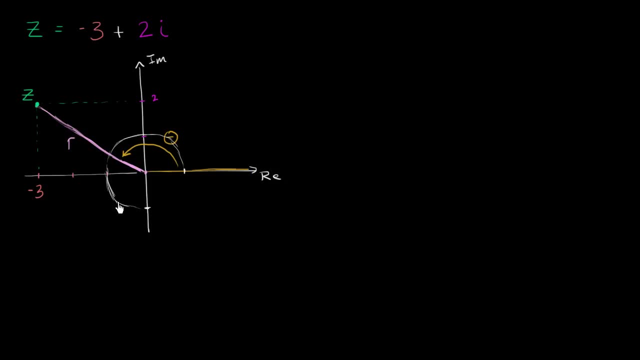 circle of radius one. So construct a unit circle. That's a unit circle By definition. what are the horizontal and vertical coordinates of this point right over here, where this line intersects the unit circle? Well, this is forming an angle of theta. 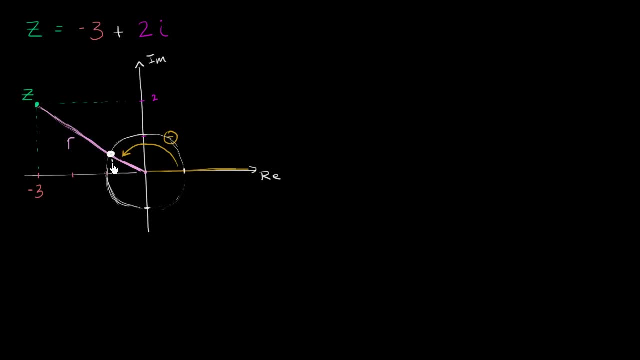 with the positive real axis, And so the horizontal coordinate over here by definition is going to be cosine of theta, cosine of theta. That's the unit circle definition of cosine of theta, And the vertical coordinate is going to be cosine of theta, to be sine of theta, sine of theta. 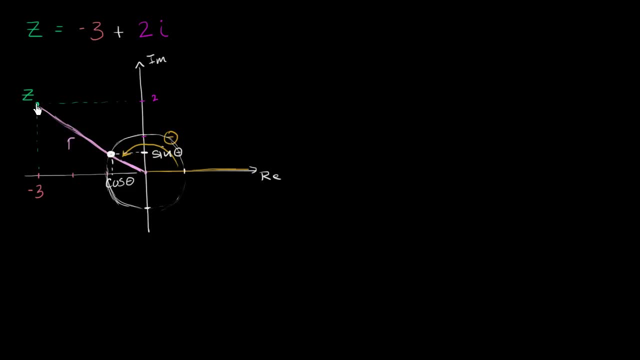 And so what would the horizontal and vertical coordinates of this point be? We obviously know they're negative three and they're two, but what would they be in terms of cosine, theta and sine of theta? Well, look this point right over here. 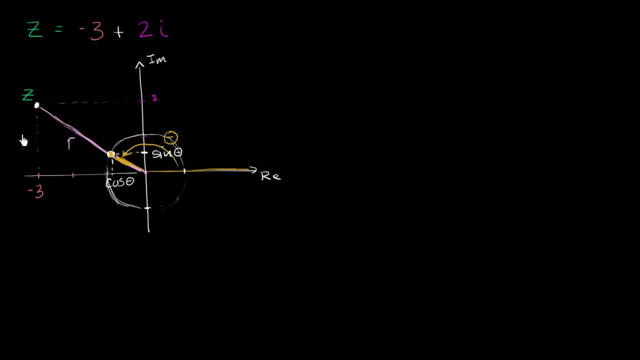 is a radius of one away from the origin. So this distance right over here, that distance right over here is one, But now we are r away from the origin. So r times as far, So for r times as far, in that direction. 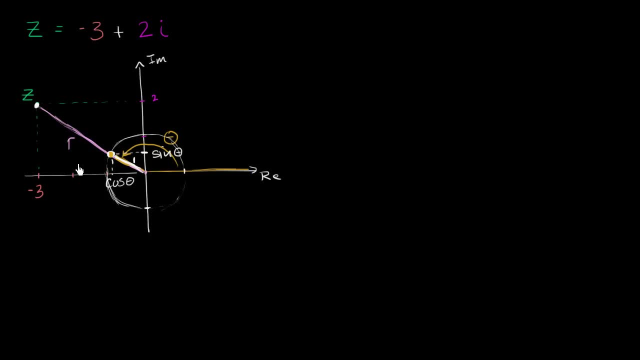 then we're going to be r times as far in the vertical direction and r times as far in the horizontal direction. We're going to have to scale all of, we're going to scale everything by r. So the horizontal, the horizontal coordinate of this point right over here. 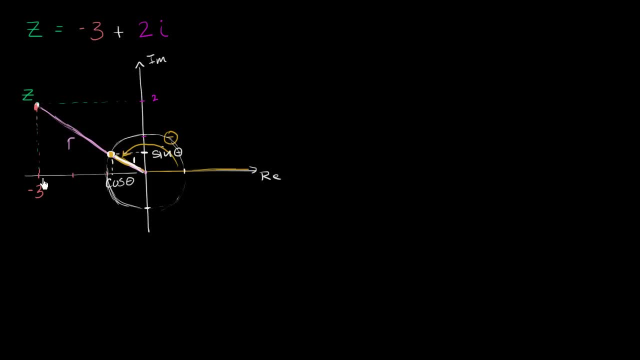 instead of it being cosine of theta, it's going to be r times cosine of theta. So this point right over here, which we know is negative three, is going to be equal to r cosine of theta. And, by the same logic, this point over here, the vertical coordinate. 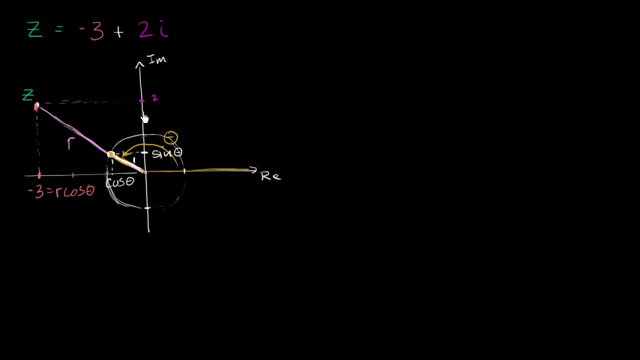 we're going to scale up sine theta by r where r times is far. So this point right over here is going to be r sine theta, And we already know that that's equal to two r sine theta. So given that, can we now figure out what r and theta are? 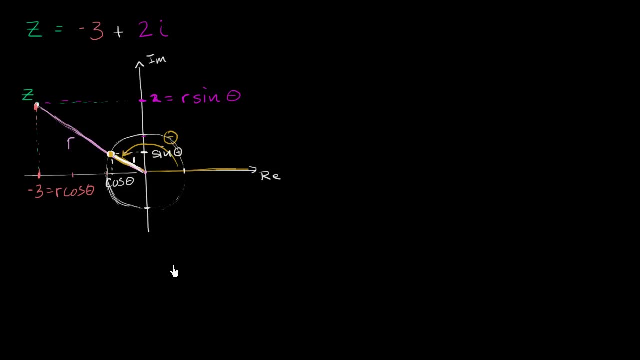 So let's first, let's first think about, let's first think about figuring out what theta is. So to do that, let's think about, let's think about some of our, our trig functions. So one, one trig function that involves: 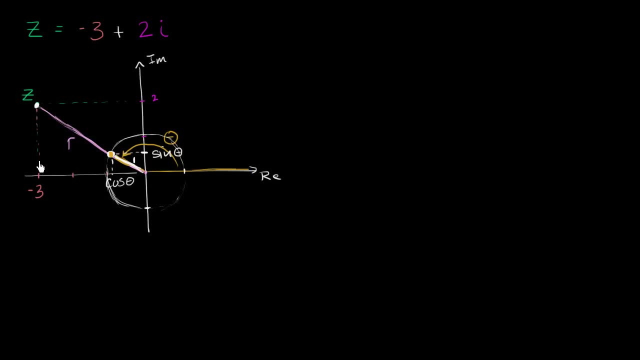 So the horizontal, the horizontal coordinate of this point right over here, instead of it being cosine of theta, it's going to be r times cosine of theta. So this point right over here, which we know is negative three, is going to be equal to r cosine of theta. 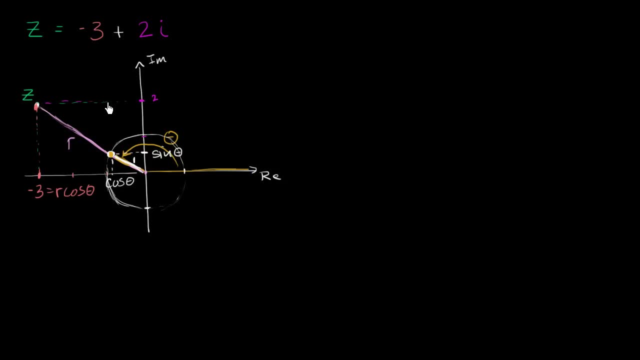 And by the same logic, this point over here, the vertical coordinate, we're gonna scale up sine theta by r, where r times is far. So this point right over here is going to be r sine theta, And we already know that that's equal to two. 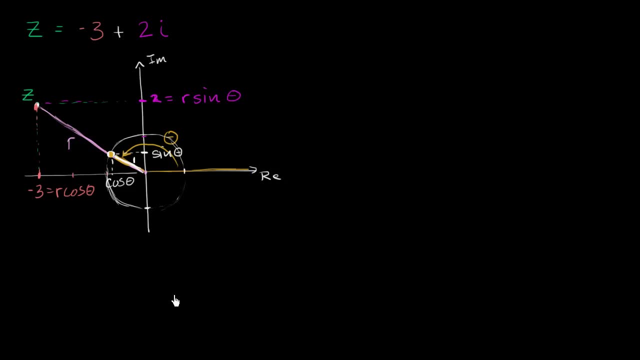 r sine theta. So, given that, can we now figure out what r and theta are. So let's first, let's first think about, let's first think about figuring out what theta is. So to do that, let's think about. 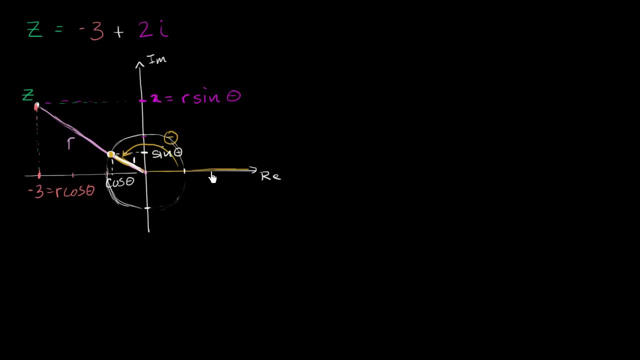 let's think about some of our trig functions. So one one trig function that involves sine theta and cosine theta is tangent theta. So for example we could say tangent theta, tangent of our angle, tangent of theta is equal to sine of theta. 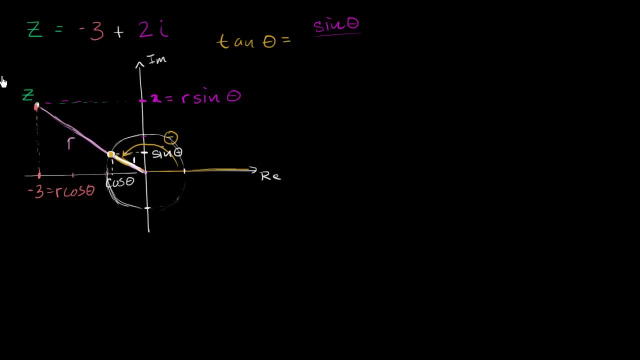 is equal to sine of theta over cosine of theta over cosine of theta. But we could also multiply the numerator and denominator here by r. that won't change the value. So that's the same thing as r sine theta over r cosine of theta. 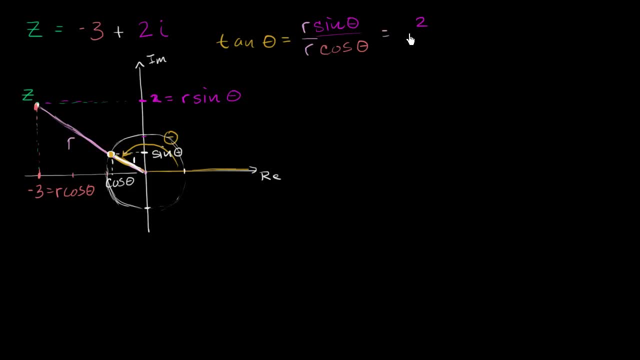 And we know r sine theta is going to be equal to two, And we know that r cosine of theta is negative three. So this whole thing is going to be negative two thirds. Another way of thinking about it is the tangent of this, tangent of theta. 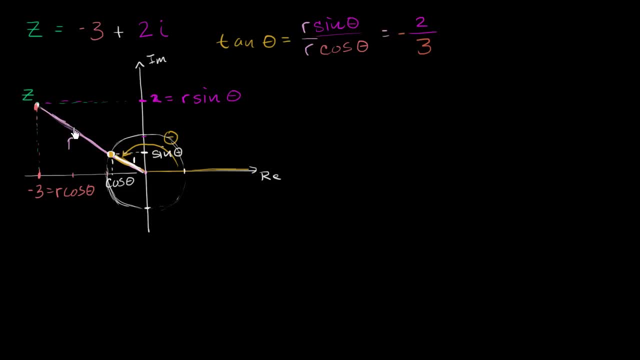 is going to be the same thing as the slope of this line right over here. And what's the slope of that line? Well, if you start at z and you want to go to the origin, you're going to go positive three in the x direction. 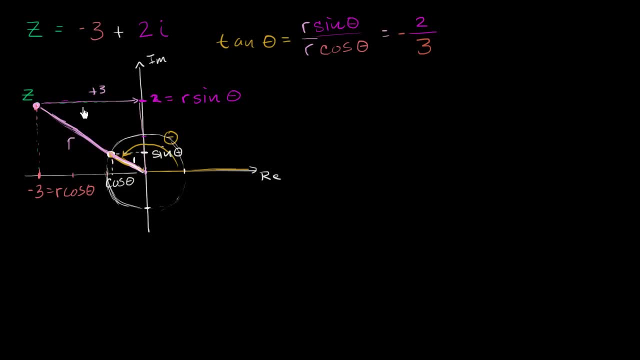 and then you're going to go negative two, or you could say positive three in the horizontal direction and then you go negative two in the vertical direction. So the slope is your change in vertical over change in horizontal. it's negative two over three. 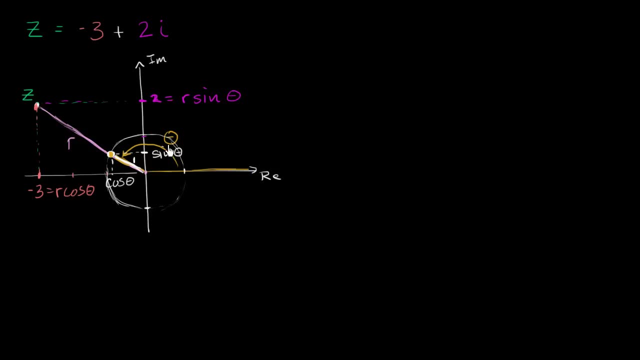 sine theta and cosine theta is tangent theta. So for example we could say tangent theta, tangent of our angle, tangent of theta is equal to sine of theta, is equal to sine of theta over cosine of theta over cosine of theta. 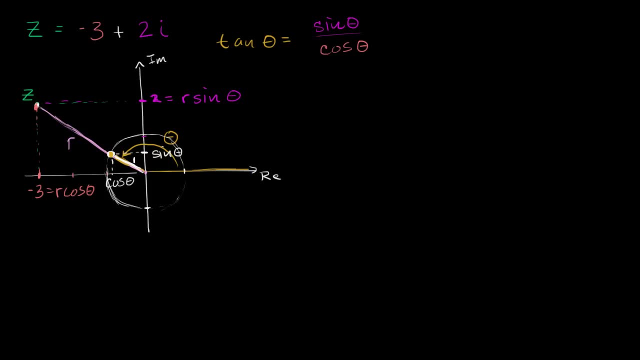 But we could also multiply the numerator and denominator here by r. that won't change the value. So that's the same thing as r sine theta over r cosine of theta, And we know r sine theta is going to be equal to two. 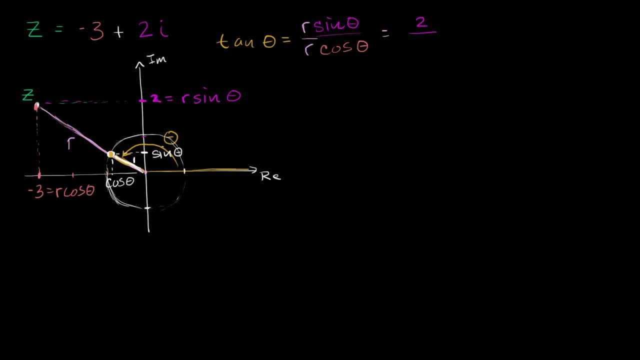 And we know that r cosine of theta is negative three. So this whole thing is going to be negative two thirds. Another way of thinking about it is the tangent of this, of tangent of theta is going to be the same thing as the slope of this line right over here. 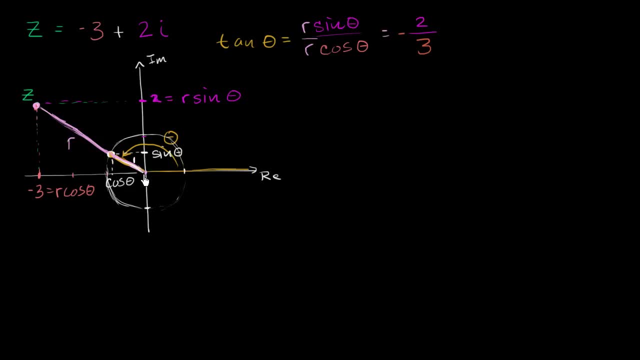 And what's the slope of that line? Well, if you start at z and you want to go to the origin, you're going to go positive three in the x direction and then you're going to go negative two, or you could say positive three in the horizontal direction. 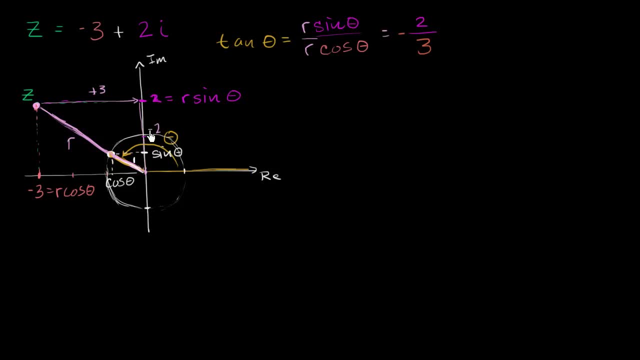 and then you go negative two in the vertical direction. So the slope is your change in vertical over change in horizontal. it's negative two over three, Negative two over three. But now we can use this to solve for theta. To solve for theta, we just take the inverse tangent of both sides. 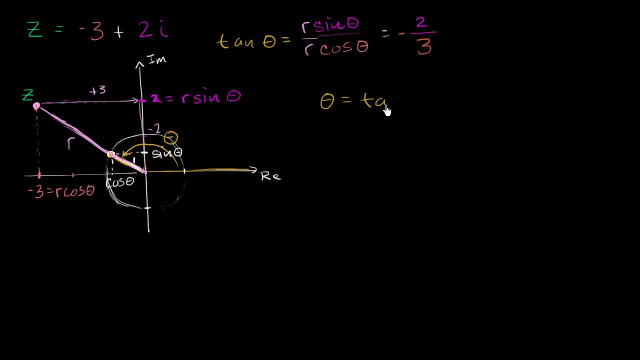 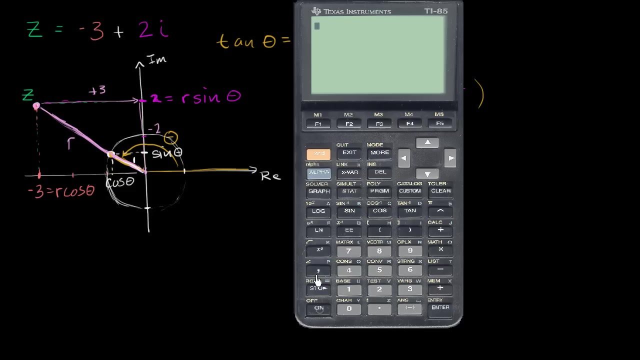 and we get: theta is equal to inverse tangent of negative- two thirds of this thing right over here. So let me copy and paste that And we can get our calculator out to figure out what this actually is. So let's turn it on. 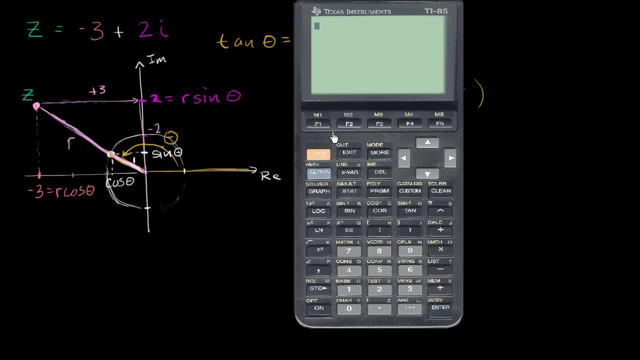 Let me make sure that I am in radian mode. I am, And so I can take the inverse tangent of negative two divided by three, which gets us negative point five, eight, eight, zero, zero, on and on and on. So if we round to the nearest hundredth of a radian, 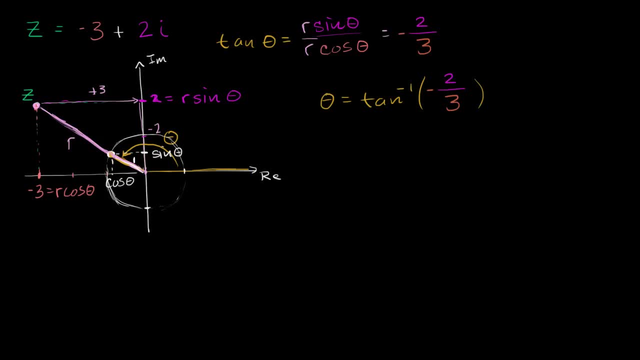 it'd be negative point five nine. So this is approximately negative zero point five nine. Now, is this the right angle? Is this the theta that we are looking for? Well, this theta- negative zero point five nine- that's going to get us over here. 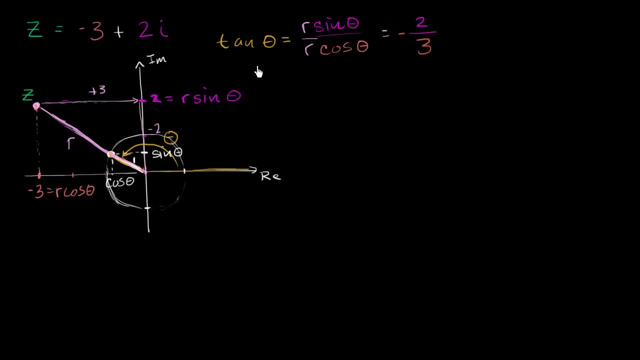 Negative two over three. But now we can use this to solve for theta. To solve for theta, we just take the inverse tangent of both sides and we get theta is equal to inverse tangent of negative. two thirds of this thing right over here. 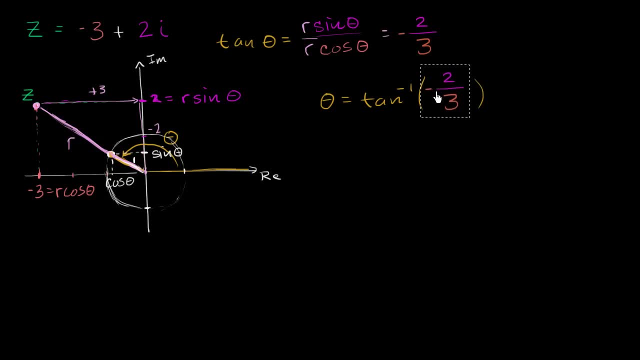 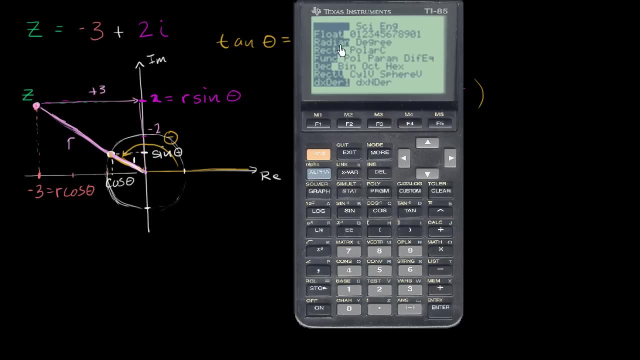 So let me copy and paste that And we can get our calculator out to figure out what this actually is. So let's turn it on. let me make sure that I am in radian mode. I am, And so I can take the inverse tangent. 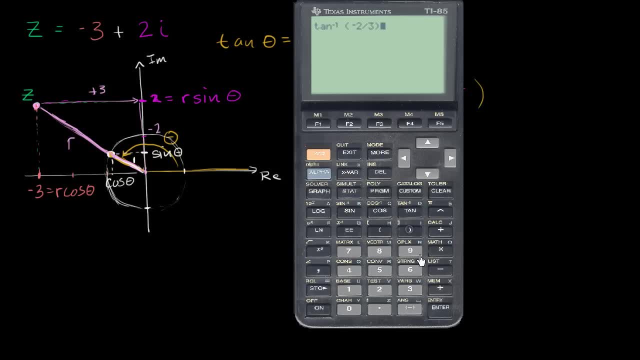 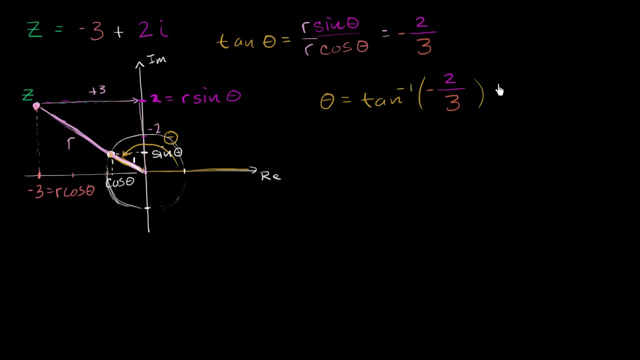 of negative two divided by three, which gets us negative point five, eight, eight, zero, zero, on and on and on. So if we round to the nearest hundredth of a radian, it'd be negative point five nine. So this is approximately. 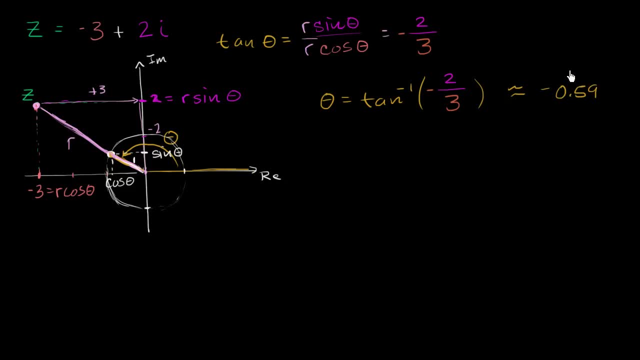 negative zero, point five, nine. Now, is this the right angle? Is this the theta that we are looking for? Well, this theta- negative zero, point five, nine- that's going to get us over here. That's this angle, Right over here. 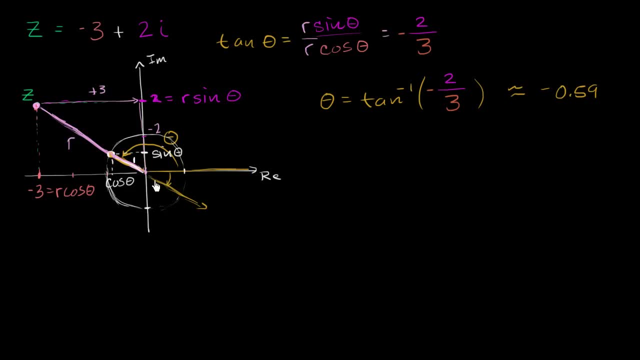 That's what the inverse tangent, that's what the inverse tangent gave us, And it makes sense, because this ray is a continuation of this ray right over here. Together they would form a line. It has the same slope, But that's not the theta that we are looking for. 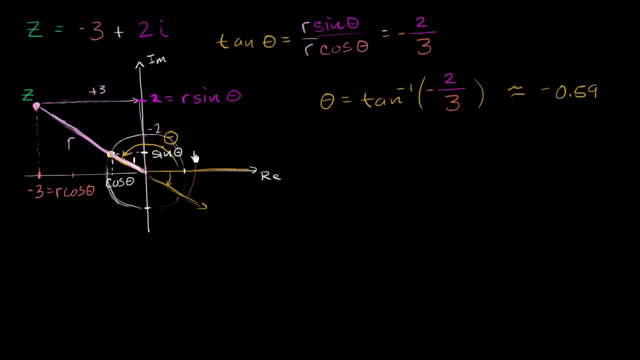 The theta that we are looking for is going in the opposite direction. It's halfway around the circle. So if we think in terms of radians, it's going to be this angle plus it's going to be this angle plus pi radians. So the theta that we are looking for 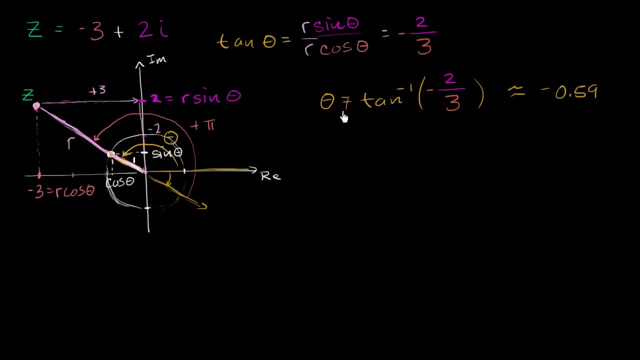 isn't zero, it isn't going to be what our calculator gives us for this. It's going to be this value plus pi. So theta- the theta that we care about- is going to be negative zero point five nine roughly plus pi. Let me say approximately, just because I have 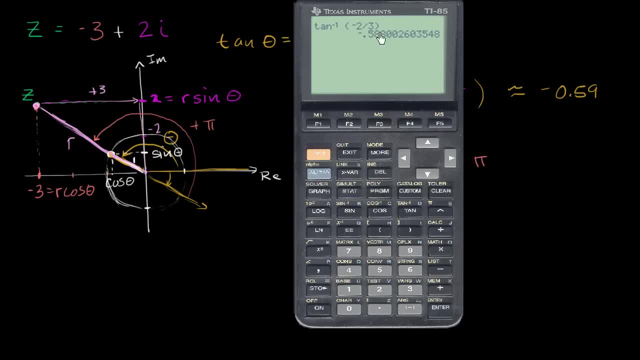 rounded right over here. So let's get the calculator out. So let's take our previous response and that's just the previous answer, Plus pi. Plus pi, because we are going to go in the opposite direction. So that gives us two point. 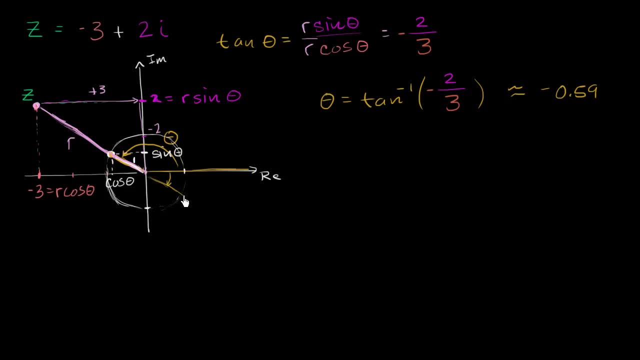 That's this angle Right over here. That's what the inverse tangent, that's what the inverse tangent gave us, And it makes sense because this ray is a continuation of this ray right over here. Together they would form a line. It has the same slope. 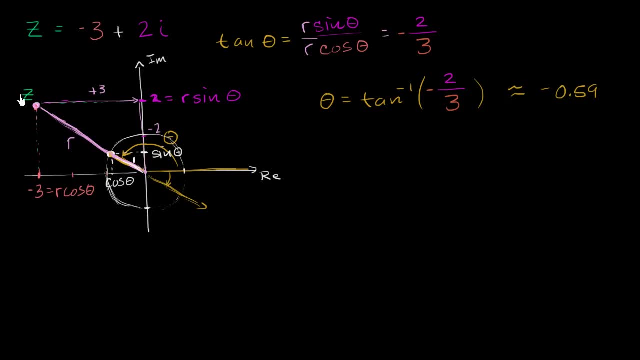 But that's not the theta that we are looking for. The theta that we are looking for is going in the opposite direction. It's halfway around the circle. So if we think in terms of radians, it's going to be this angle plus. 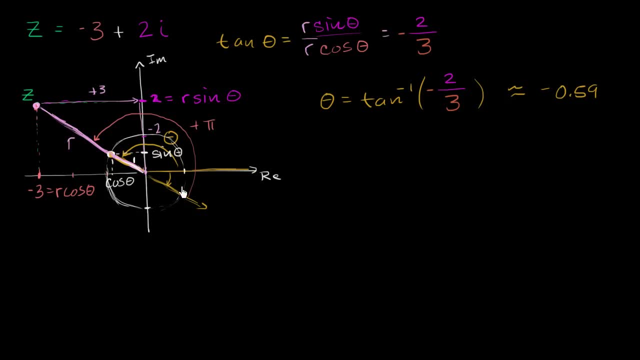 it's going to be this angle plus pi radians. So the theta that we are looking for isn't zero, it isn't going to be what our calculator gives us for this. It's going to be this value plus pi. So theta, the theta that we care about. 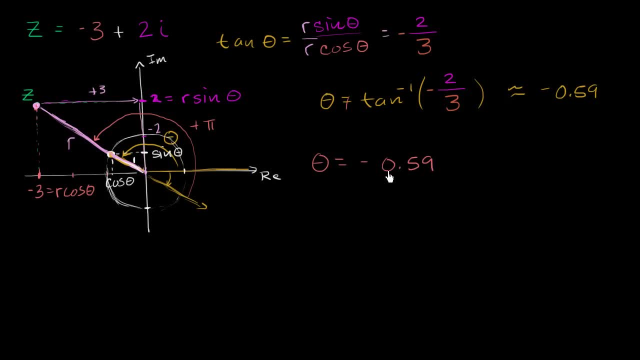 is going to be negative zero point five nine roughly plus pi. Let me say approximately, just because I have rounded right over here. So let's get the calculator out. So let's take our previous response and that's just the previous answer. 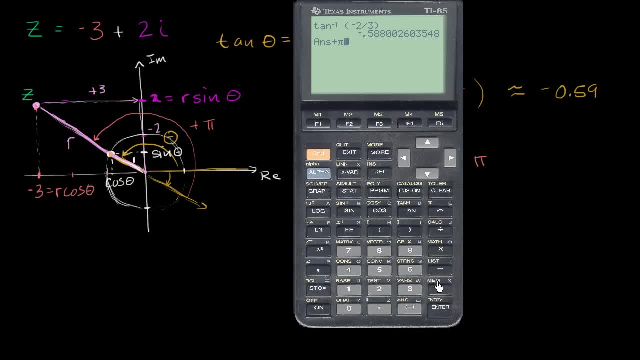 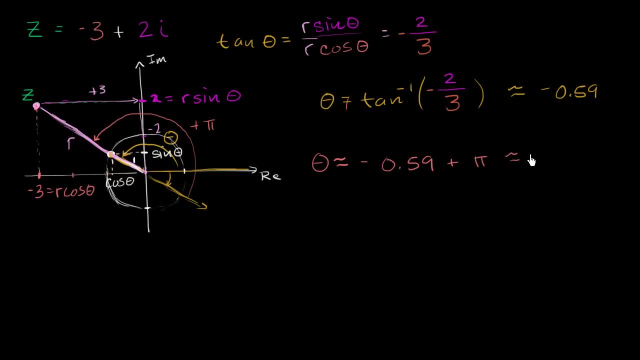 plus pi. Plus pi because we are going to go in the opposite direction. So that gives us two point, roughly two point five five radians. So this is approximately two point five, five radians is our claim for what theta is. Now, does that make sense? 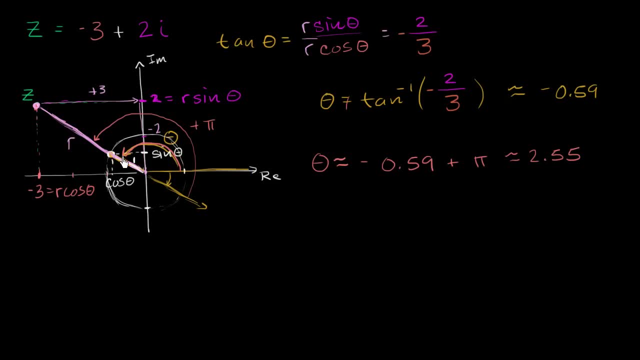 that this angle, that this angle right over here, is two point five, five radians. Well, this angle, if we go straight up, that's pi over two radians And pi is three point one four, so that's going to be one point five seven. 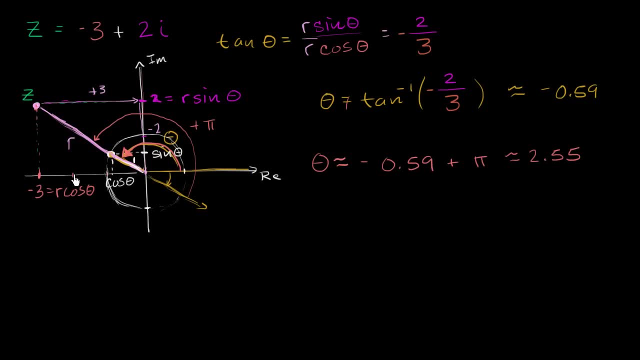 right, one point, something like that, And this is pi radians. so that's three point one, four, one, five, nine keep going on and on and on. So two point five, five is indeed in the right quadrant, So that is right. 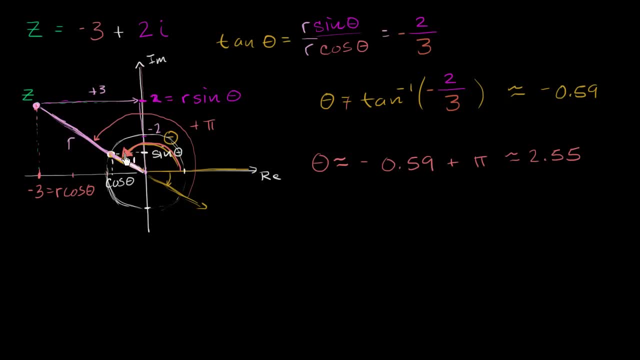 This is going to be an angle of two point five, five radians. Now we just have to figure out the length, what r is, And that we can just use the Pythagorean theorem, for We could set up a right triangle, a right triangle. 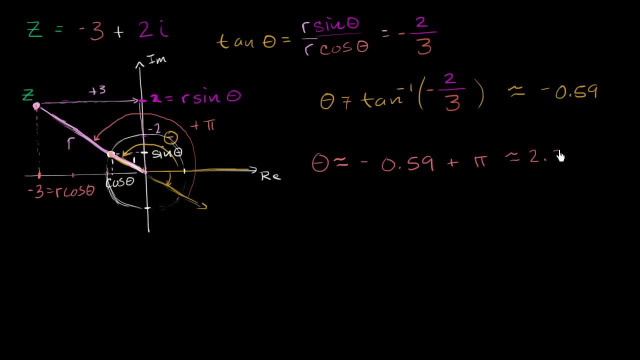 roughly two point five, five radians. So this is approximately two point five, five radians, is our claim for what theta is Now. does that make sense that this angle, that this angle right over here is two point five, five radians? Well, this angle, 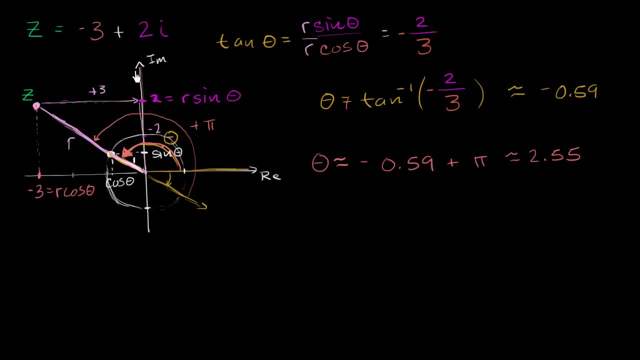 if we go straight up, that's pi over two radians. So that's going to be one point five, seven, right, one point, something like that. And this is pi radians. so that's three point one, four, one, five, nine. keep going on and on and on. 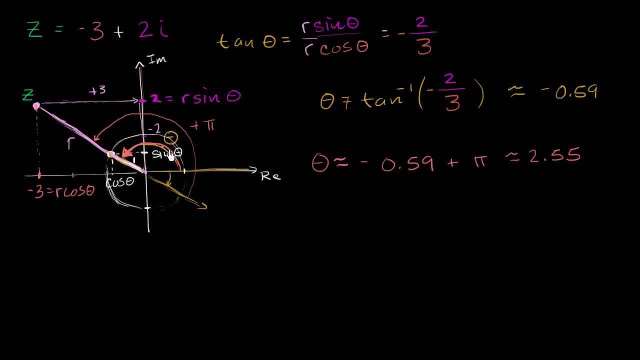 So two point five five is indeed in the right quadrant. So that is right. This is going to be an angle of two point five five radians. Now we just have to figure out the length, what r is, And that we can just use the Pythagorean Theorem for. 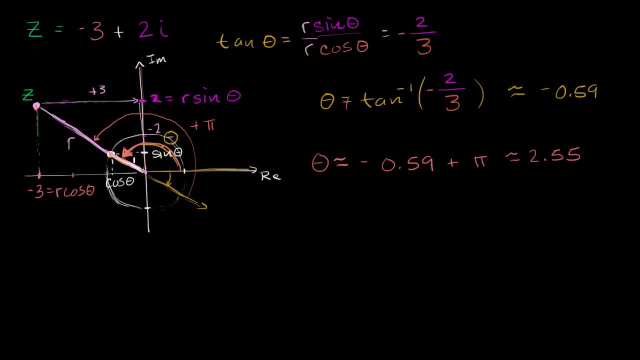 We could set up a right triangle, a right triangle, a right triangle. we know that this distance, this distance right over here is two, because this distance right over here is two, And we know that this distance, this distance is the coordinate here- is negative three, but the distance here is just three. 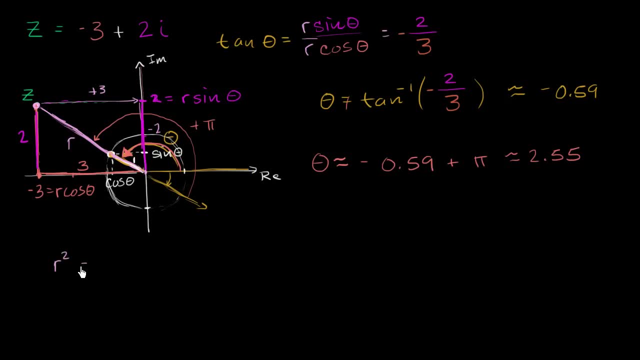 So we know from the Pythagorean Theorem that r squared is equal to two, squared is equal to two squared plus three, squared plus three squared, Or that r is equal to the square root of four plus nine, which is thirteen. And so there we have it. 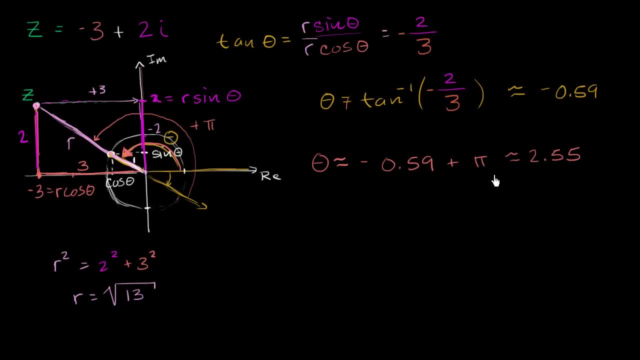 We have negative three. So we know that r is equal to the square root of thirteen and theta is two point five, five radians. So using that information, we can now rewrite z in terms of r and our theta. So now can say that z is equal to, instead of negative three. 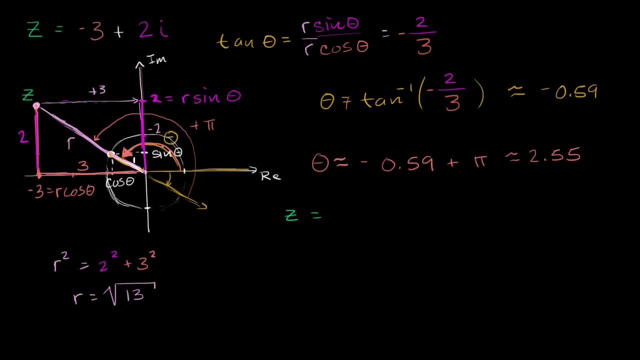 we can write it as r cosine theta, so we can rewrite it as square root of 13 times the cosine of theta, which is, we're saying theta is roughly 2.55. if we round to the nearest hundredths plus 2, we already know is r sine of theta. 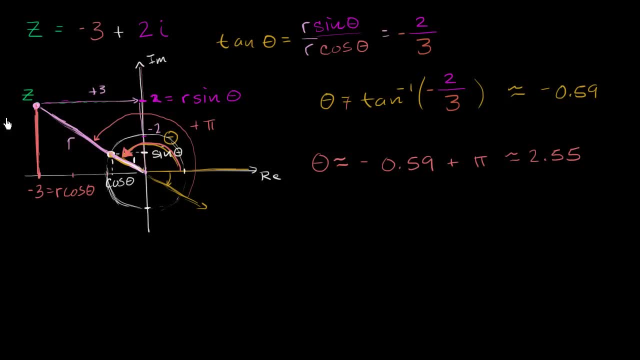 We know that this distance, this distance right over here, is two, because this distance right over here is two, And we know that this distance, this distance is the coordinate here- is negative three, but the distance here is just three. So we know from the Pythagorean theorem: 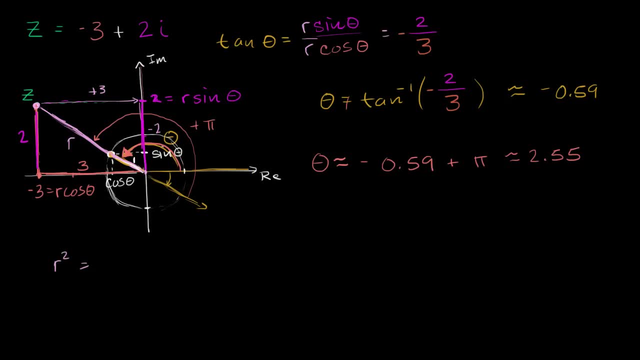 that r, squared, is equal to two squared is equal to two squared plus three squared plus three squared, or that r is equal to the square root of four plus nine, which is thirteen. And so there we have it. We have negative three. 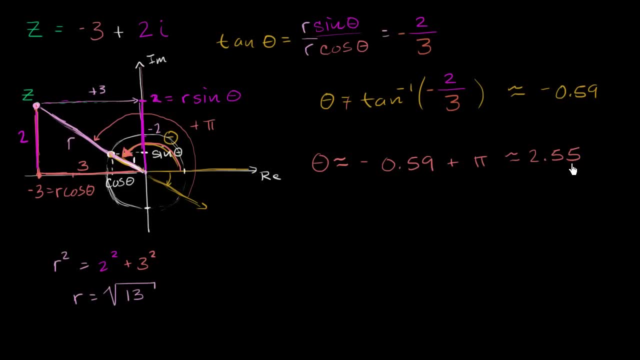 so we know r is equal to the square root of thirteen and theta is two point five, five radians. So using that information, we can now rewrite z in terms of r and our theta. So now we can say that z is equal to. 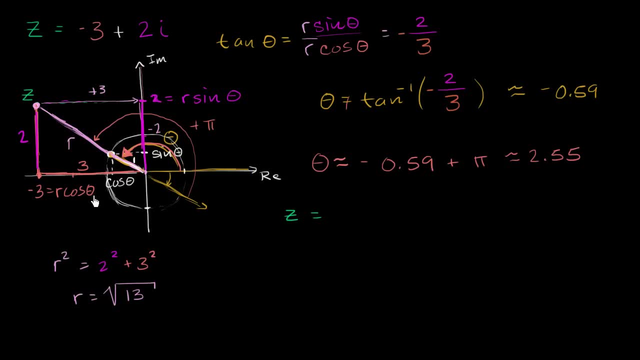 instead of negative three we can write it as r cosine theta, So we can rewrite it as square root of thirteen, square root of thirteen times the cosine times, the cosine of theta, which is we're saying. theta is roughly two point five five. 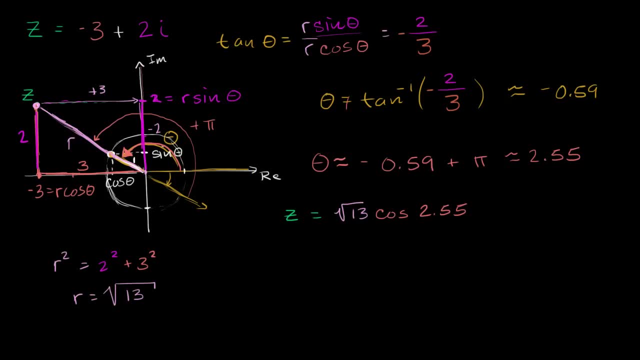 if we round to the nearest hundredths plus plus two, we already know, is r sine of theta. So r is square root of thirteen, square root of thirteen, and then sine sine of theta, two point, five, five, and then all of this we could say: 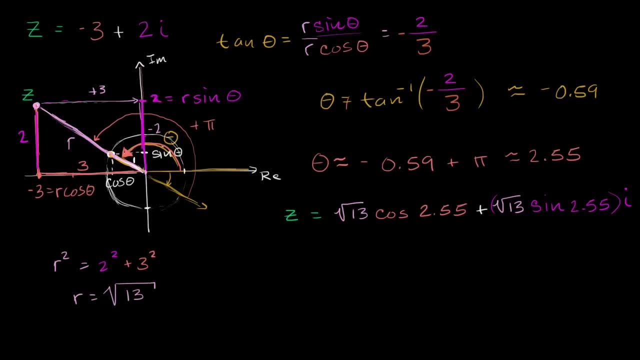 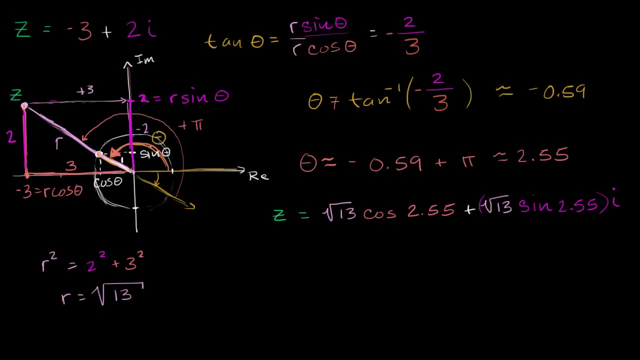 or all of this is going to be multiplied times i, And if we like to simplify it a little bit or kind of really make clear what the r is here, we could factor it out. So we could say that z is equal to square root of thirteen. 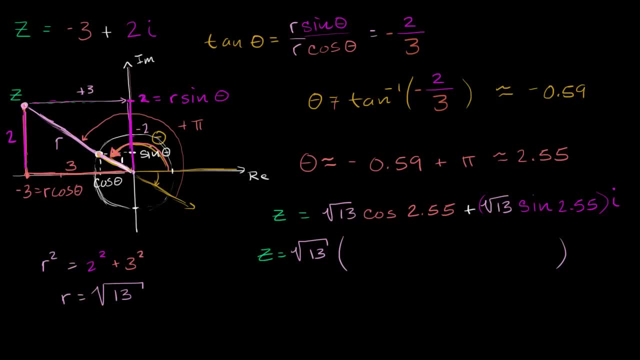 square root of thirteen times cosine of two point five five. and once again, two point five five is an approximation, so maybe I should say approximately equal to cosine of two point five five, cosine of two point five five plus plus. 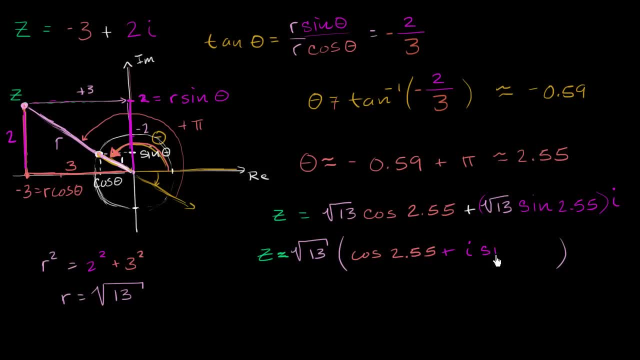 I'll throw the i in front, plus i times sine of two point five, five, And so when I rewrote z in this format right over here, it makes it much clearer what the direction I have to go in is. the direction is two point five, five radians.